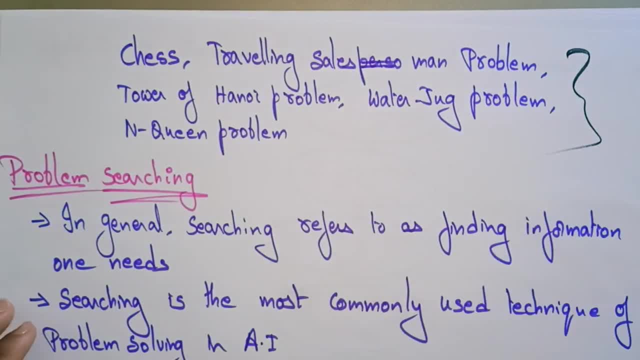 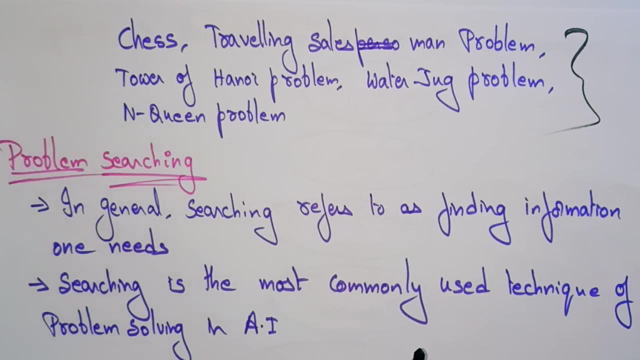 problem, water jet problem and queen problem. So these are all based on the artificial intelligence. So most of the problem solving exam Examples techniques with the help of artificial intelligence. So these are, everything is based on artificial intelligence. Now coming to problem searching. So why I'm talking about the problem? 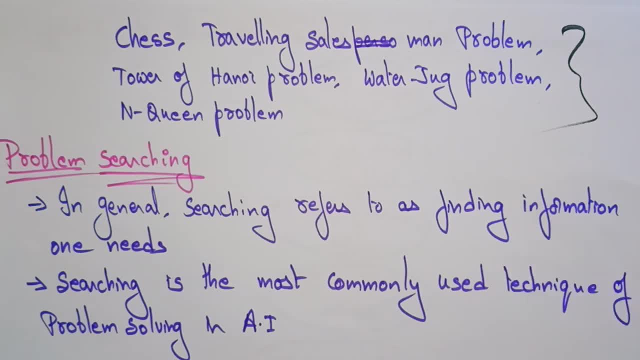 searching. So now I'm talking about the problem solving. Again. I skipped into problem searching. What is this problem searching? In general, searching refers to as finding information. one needs that. we know that when you will search if you want to find some information that you needed. 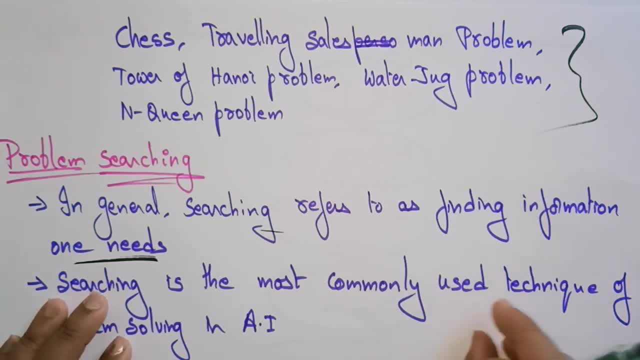 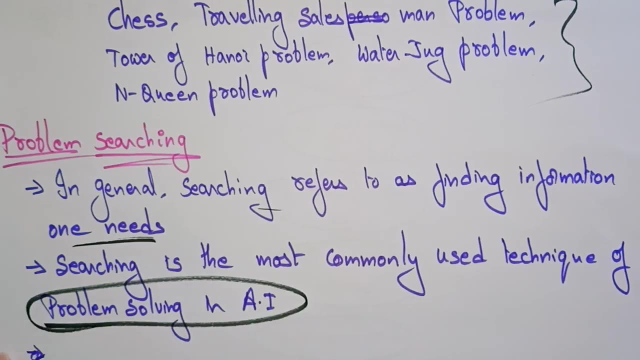 that is a searching technique. I'm searching for my page. where is my page exactly? suppose 25 is my page. I'm searching for that 25 page. So in general the searching is like that: finding information one needs. So searching is the most commonly used technique for problem solving in AI. That's why I'm 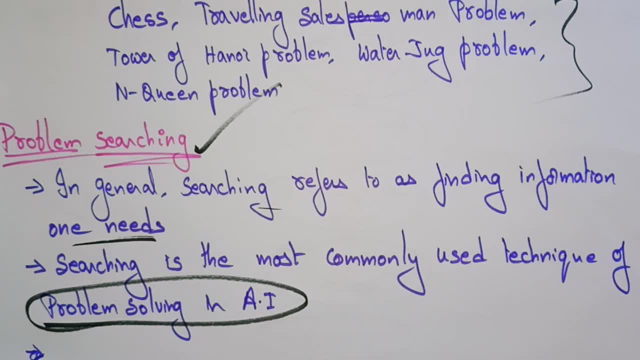 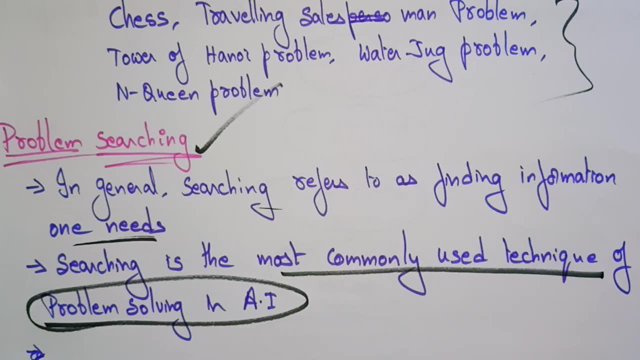 talking about the problem searching, Because this searching is the most commonly used technique of problem solving and artificial intelligence. In artificial intelligence, if you want to solve, if you to do the problem solving concept, okay, then you will use the technique searching, not only the. 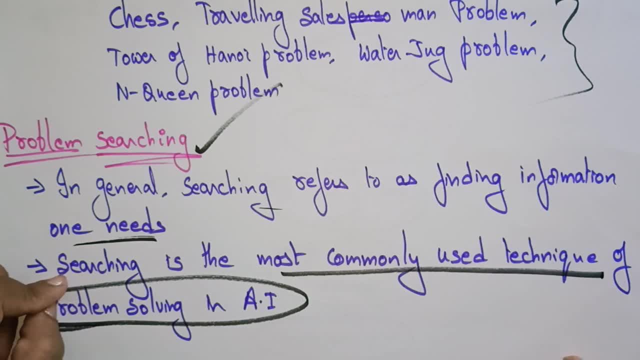 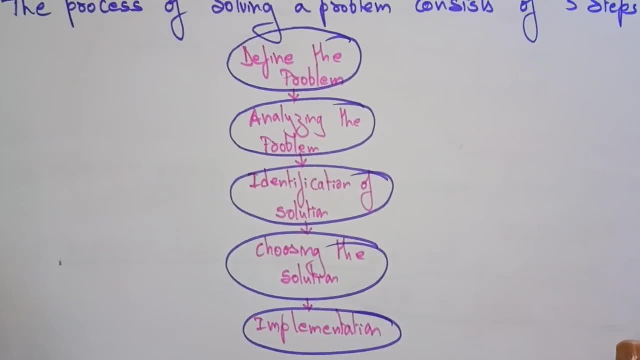 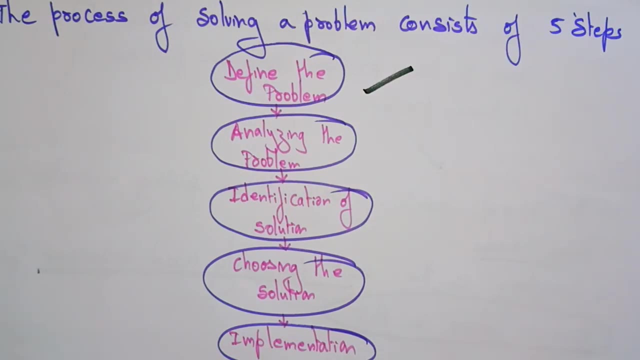 searching. another type of methods will be there, but searching is a most commonly used technique of problem solving in artificial intelligence. so what are the steps that you have to follow for solving a problem? first thing is you have to define the problem. what is your problem? okay, what you are going to be find out by using the artificial intelligence, okay i'm. i want to find. 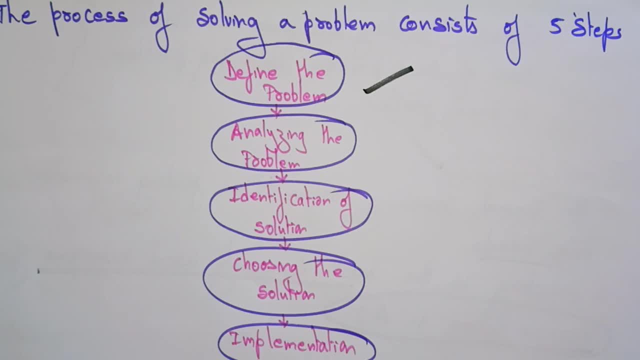 out: uh, i'm my agent, is i? i want to create an self-driving car. okay, i want to create a chess uh game in my system. i want to create one pseudocode game in my system. so first is you have to define the problem: what, what you are going to be designed. next, analyze the problem. 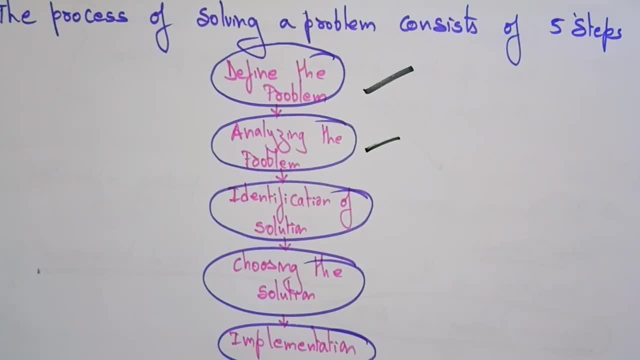 means what are the different conditions that you have to be taken? what to solve that problem? okay, it's a here the problem means it is not a drawback. you are going to find something that is a problem solving if something is there in your mind, if you try that.